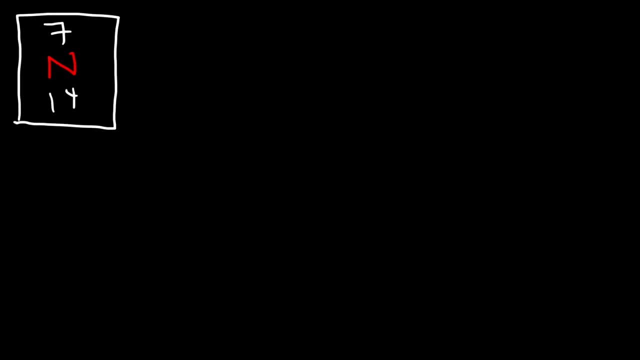 number, and the smaller of the two numbers is the atomic number, which is an integer. Now, what you need to know is that in the first energy level, you have the 1s sublevel. In the second energy level, you have the s and the p sublevels, In the 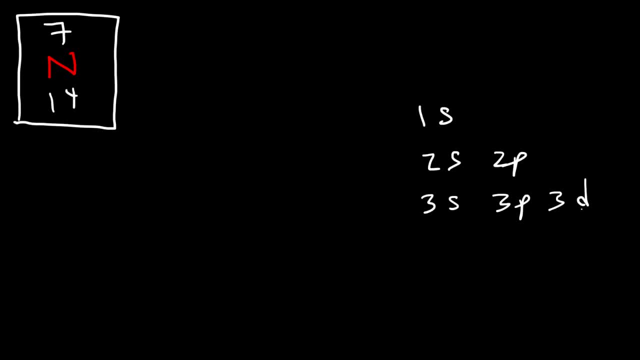 third energy level. you have s, p and d. Now for nitrogen. this is as far as we need to go. The s sublevel can hold two electrons and the p sublevel can hold six and d can hold ten. Now you want to write the electron configuration until you get a total of. 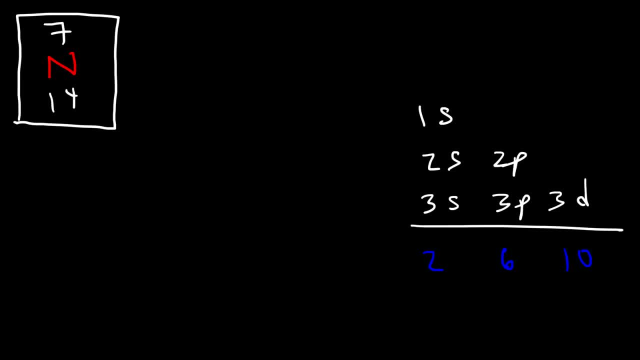 seven. Now for an atom of nitrogen. it contains seven protons and seven electrons, but we're focused on the number of electrons because we're writing the electron configuration. For ions that number could differ, but for atoms you just need to focus on that number. So the number of electrons in this problem is: 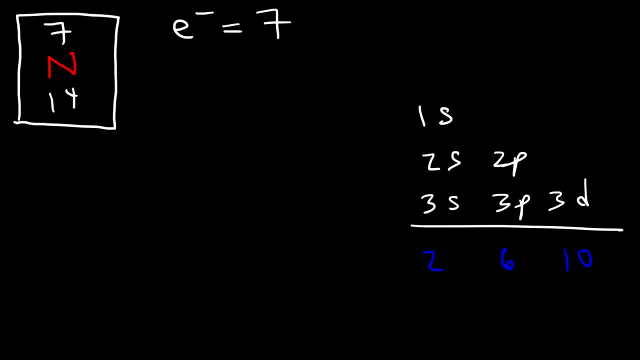 seven. So here's what we need to do. First, start with 1s. So I'm going to write 1s2, because s can hold up to two electrons. Next move on to the 2s sublevel. 2s can also hold two. 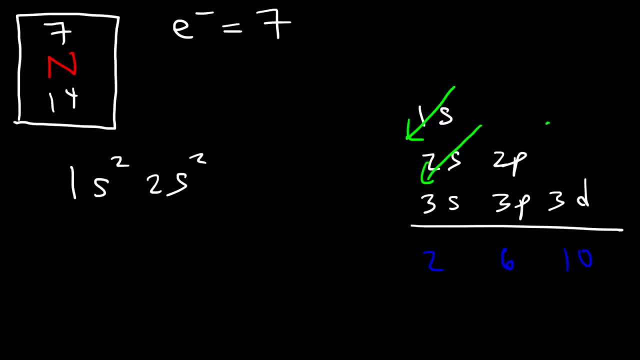 electrons, And then after 2s you want to go to 2p and then 3s. Now 2p can go up to six. It can hold six electrons, but we only need three more, because if you add the exponents two plus two plus three is seven. 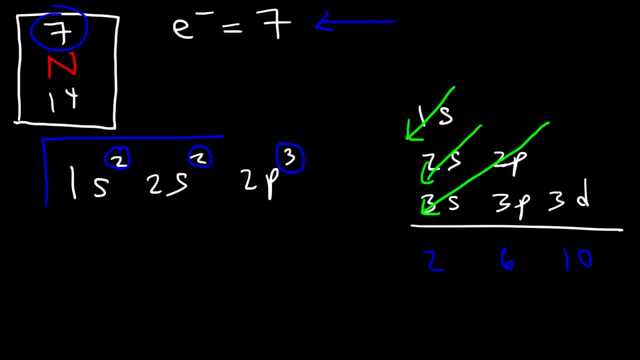 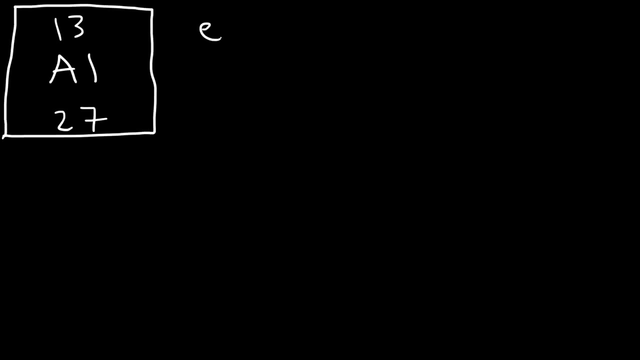 Once you get up to this number for atoms, you can stop. This is the electron configuration for an atom of nitrogen. Now let's try another example. Let's write the electron configuration for aluminum. You could try if you want to. So we're dealing with an atom of aluminum which has 13 electrons. So you: 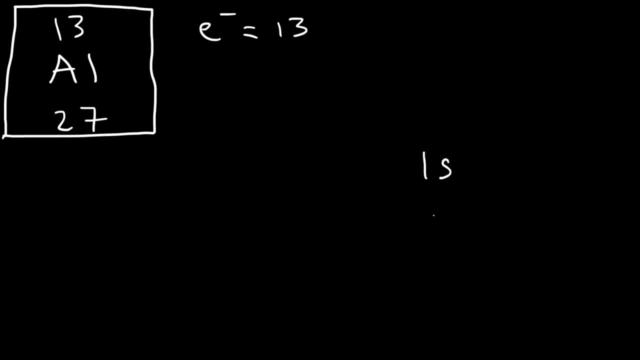 want to write the configuration up to 13.. Now, we're going to set it up the same way. Now, if you want to, you can add the fourth energy level, which contains 4s, 4p, 4d and 4f. Now let's put these numbers. 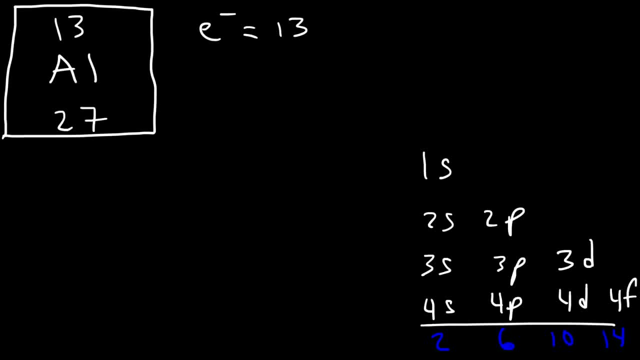 again, F can hold up to 14 electrons, So we're going to start with 1s, So that's 1s2.. And then, after 1s, we have the 2s sublevel, So this is going to be 2s2.. 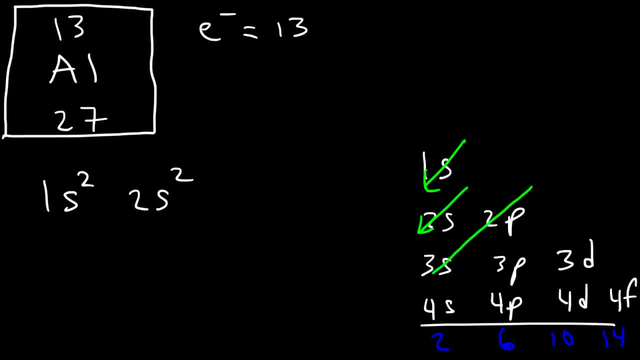 And then we need to move on to 2p, then 3s, So p can hold up to 6 and s can hold up to 2.. So if we add the numbers 2 plus 2 plus 6 plus 2, that's 12.. We only. 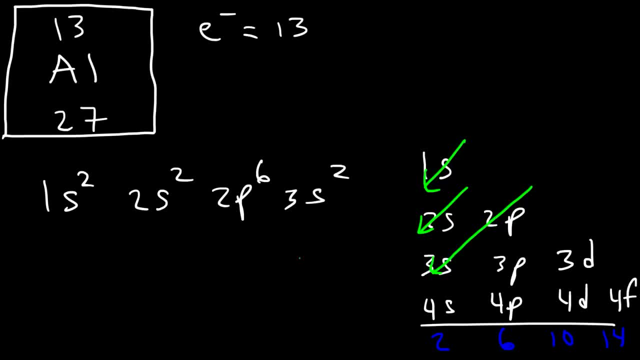 need one more. So after 3s we need to move on to 3p. Now we don't need to go up to 3p6. We only need one more. So we're going to stop at 3p1.. So if you add 2, 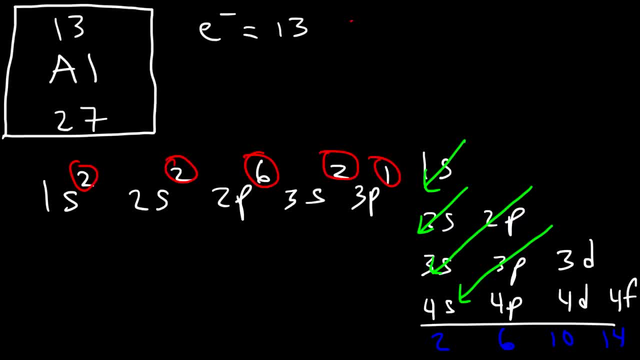 plus 2 plus 6 plus 2 plus 1, that will give you 3p6.. So if you add 2 plus 2 plus 6 plus 2 plus 1, that will give you 3p6. a total of 13.. So this is the ground state electron configuration of an atom. 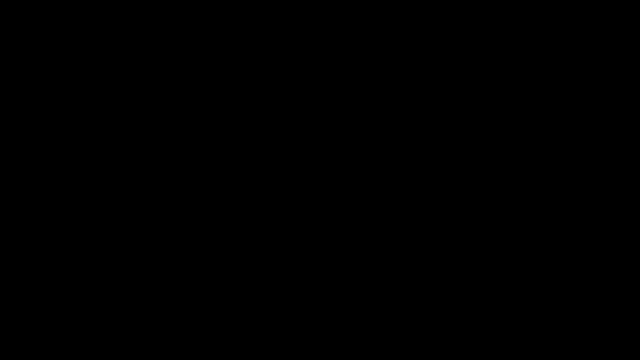 of aluminum. Now what about ions? Let's say, if we want to write the electron configuration of the Fe2 plus ion, How can we do so? Now? on a periodic table, Fe has an atomic number of 26 and an average atomic mass of about 55.85.. 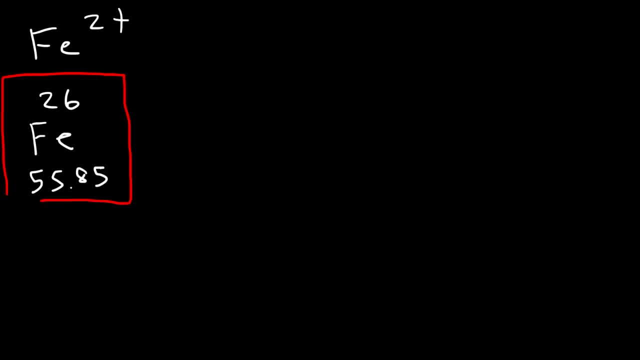 So an atom of iron metal has 26 electrons. So what about an ion of Fe? Because the charge is plus 2. that means that the atom lost two electrons. So therefore the Fe plus 2 ion has 24 electrons. It has two less than this. 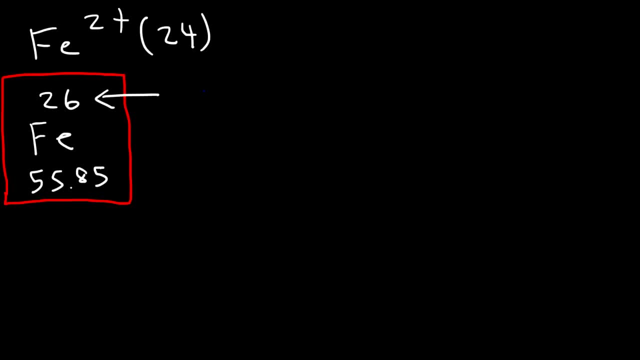 number. So we're going to write the electron configuration based on the number 24.. So let's make our list again: 1s, 2s, 2p, 3s, 3p, 3d, 4s, 4p, 4d, 4f. 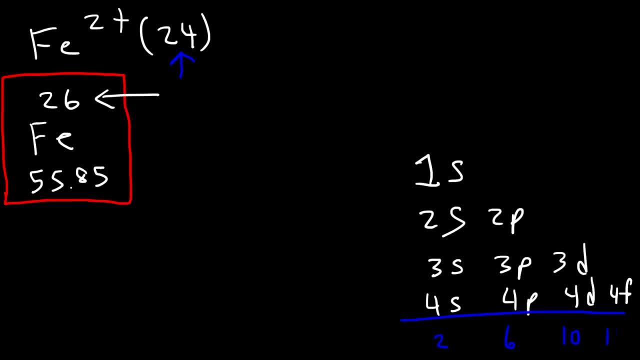 s can hold 2, p can hold 6, d can hold 10, f can hold 14.. So we're going to start with 1s, So that's going be 1s, 2, and then we'll move onto 2s. So let's THE eyes day right. Make sure the hold only at 3s, so we've going to pick 5s. then we bring 4anout2.. avoiding the animalssek. So this is going to be 2s2.. 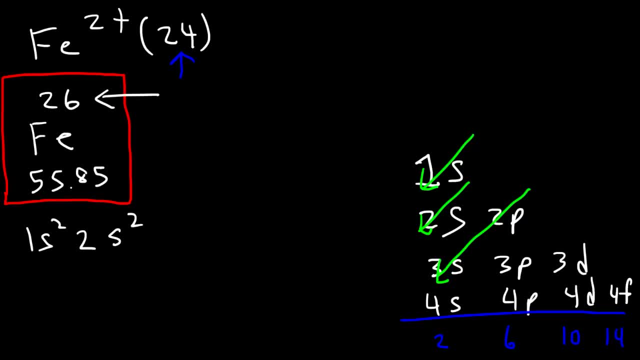 And then we're going to go to 2p, then 3s, So it's going to be 2p6, and then 3s2.. Now, after 3s, we've got to move on to 3p, then 4s. 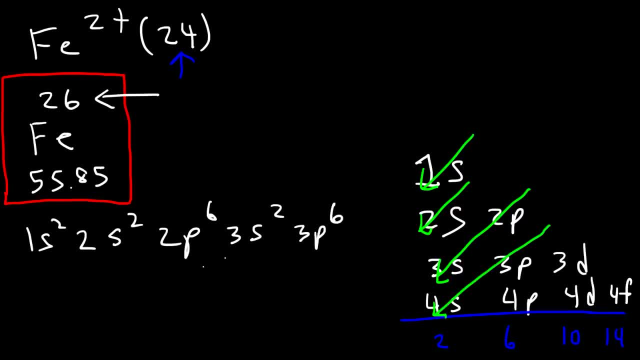 So it's 3p6, and then 4s2.. By the way, before you write the electron configuration of Fe plus 2,, it's better if you write the electron configuration of the parent atom And then from that write the electron configuration of the ion. 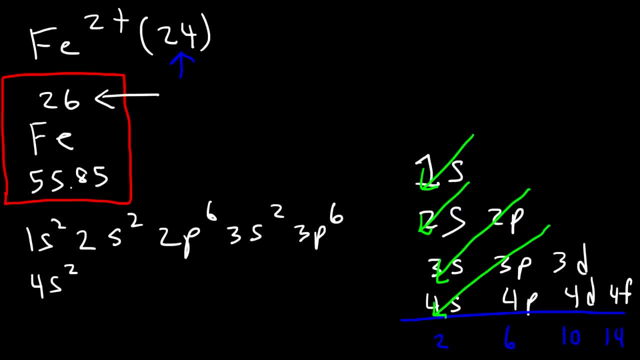 So I'm going to focus on 26, and then I'm going to adjust it to 24.. So right now we have a total of 2 plus 2 plus 6 is 10.. 2 plus 6 plus 2 is another 10.. 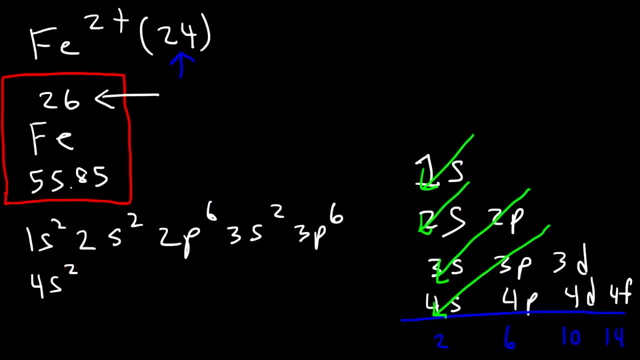 So we need 6 more electrons to get to 26.. So after 4s comes the 3d sub-level. Now d can hold up to 10,, but we only need 6 more. So this is the electron configuration of Fe, but not Fe plus 2.. 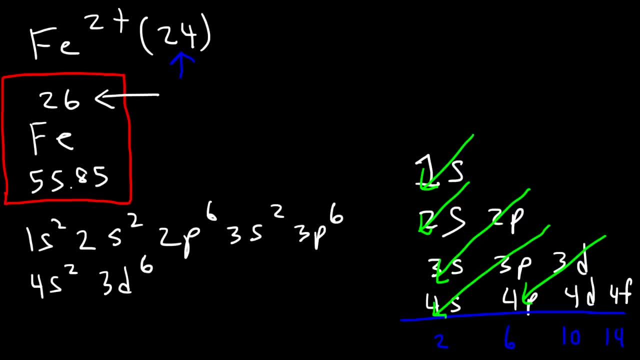 Because we have a total of 26 electrons. Now, from this expression you want to write the electron configuration of Fe 2 plus, So you need to remove 2 electrons. The question is, which 2 electrons do you remove? Now, what you need to do is remove electrons from the highest energy level. 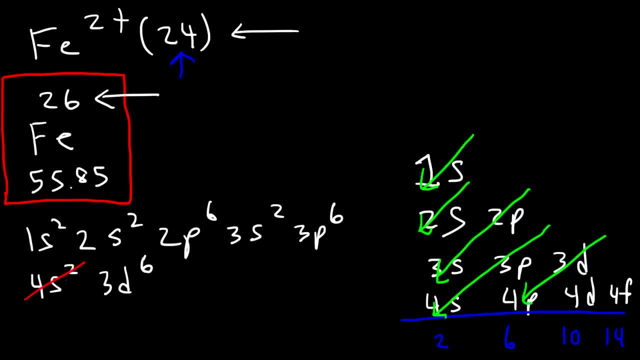 So that's from the 4th energy level. So you're going to take off these 2 electrons. So we could therefore write the configuration for Fe 2 plus as 1s2, 2s2,, 2p6,, 3s2,, 3p6, 4s0,. or you could just omit it and then 3d6.. Now if you were to write the configuration based on this number, and if you didn't do this step first, you might be inclined to write 4s2,, 3d4, and it won't be correct. 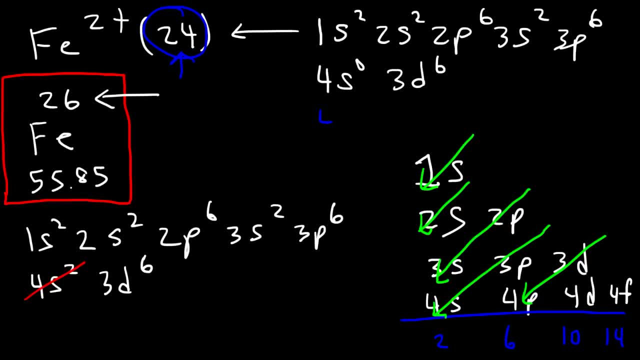 So when you're dealing with transition metal ions, it's best to write the configuration of the parent atom first and then, if you have a positive charge, simply take off electrons. that's equal to the charge starting from the highest energy level. 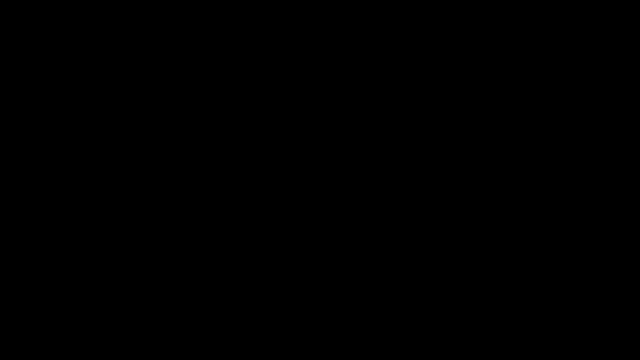 Now let's move on to our next example. So we're going to deal with chlorine. So here's the information that you need to know for chlorine. Now what I want you to do is write the electron configuration for the chloride ion. Go ahead and try that problem. 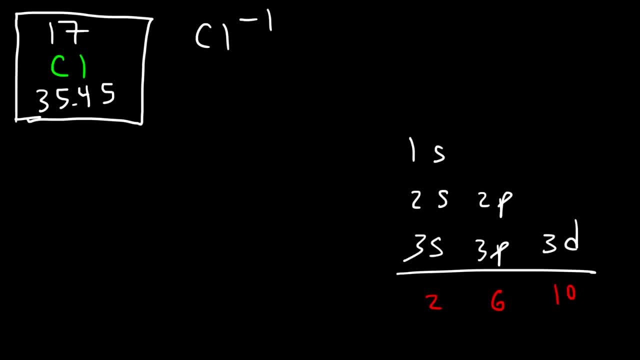 Now for chlorine. we really don't need the fourth energy level, So let's start with this. We need to get up to 17, and then we're going to add one. Chloride has a total of 18 electrons. Now for this one, we can just go straight to 18.. 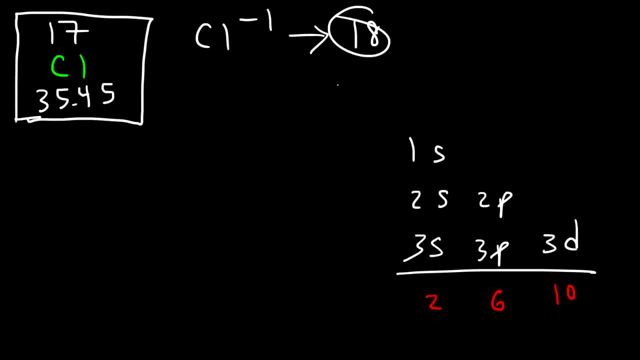 We don't have to start from 17 and add one. You could do that if you want to, but you don't have to because chlorine is not a transition metal. So I just want to read this. I just want to rephrase this one more time: 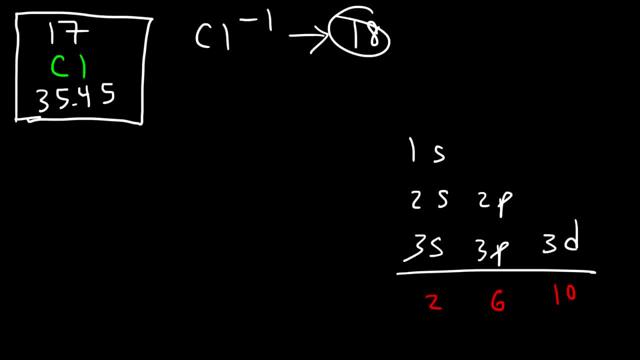 For transition metals, it's best to write the electron configuration first and then subtract the appropriate number of electrons based on the charge For elements that are not transition metals, and if you're dealing with ions you can go straight to this number. 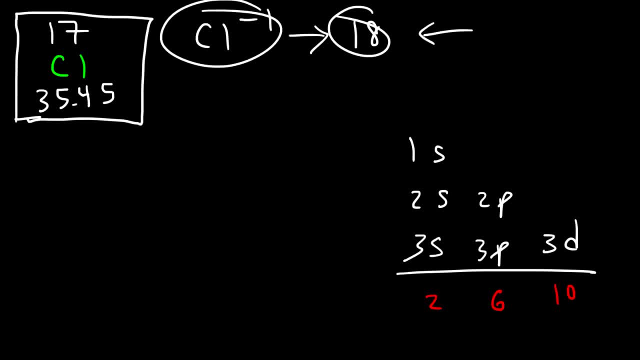 You could find the total number of electrons in the ion and then write the configuration. based on that. You don't have to write the configuration of the atom and then adjust it for the ions. It'll just simply work out that way, but you could do it both ways for these elements. 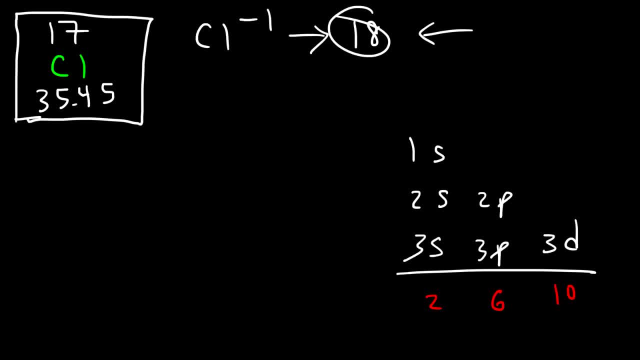 So if you decide to write the electron configuration for the parent atom and then adjust it for the ions, then that's fine. For negatively charged ions you need to add electrons. For positively charged ions you need to subtract the electrons. So let's start. 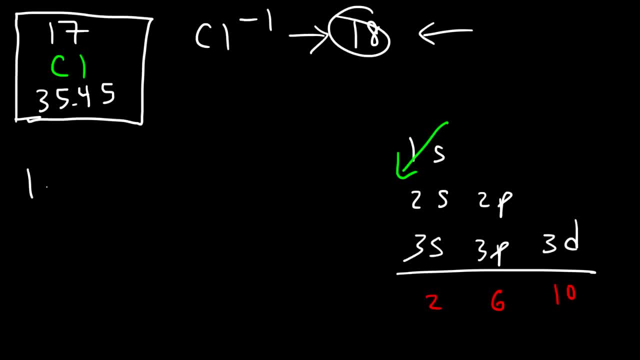 We need to get up to 18.. So we're going to start with 1s. So this is going to be 1s2.. And then it's going to be 2s2.. And then it's going to be 2s2.. 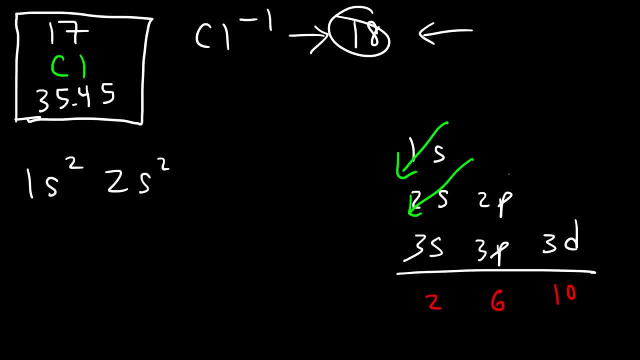 And then it's going to be 2s2.. After 2s comes 2p, then 3s, So it's 2p6, and then 3s2.. So far we have a total of 12, so we need 6 more.